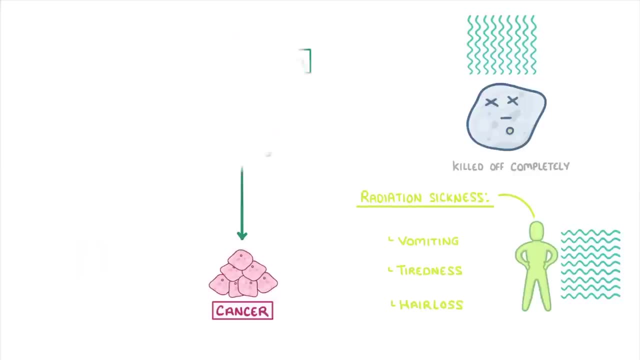 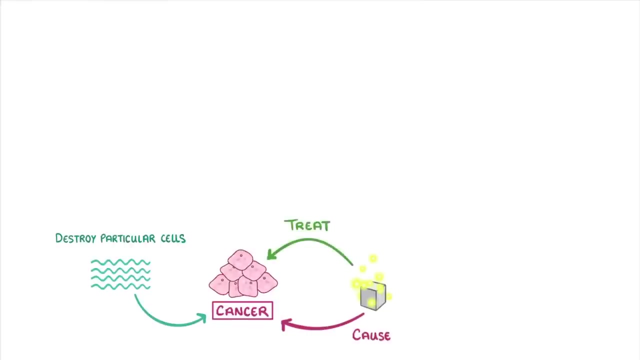 really ill. On the bright side, doctors can use this radiation to destroy particular cells that we don't want, like cancer cells. Although radiation radiation can cause cancer, it can also treat cancer. We call this process radiotherapy, and there are two main ways that we can deliver the radiation: externally or internally. External: 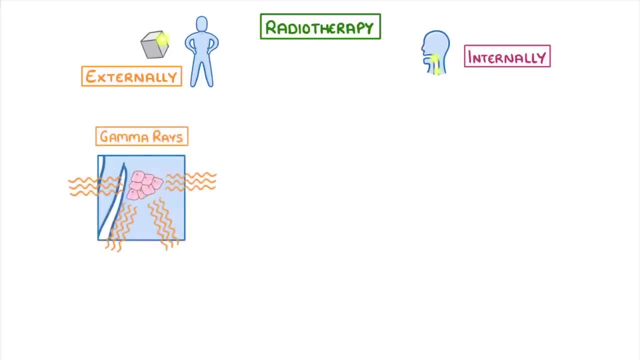 sources normally emit gamma rays that are targeted at the cancer site from lots of different angles, so that only the cancer site gets the highest dose. The internal method is where we place the radioactive source inside the body, either inside the cancer itself or next to the cancer. This method usually uses beta radiation, which is more damaging than gamma. 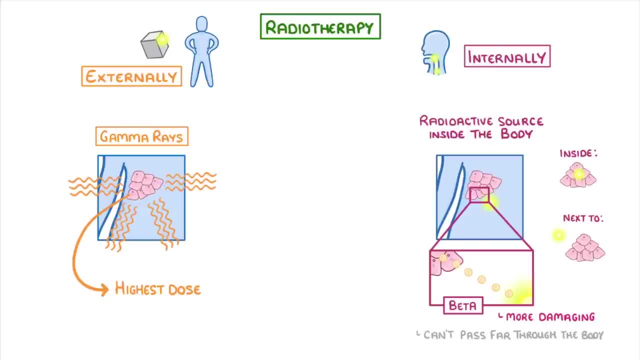 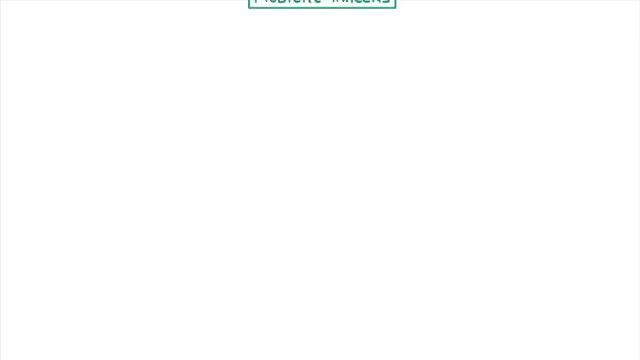 rays but can't pass as far through the body. Unfortunately, both of these techniques have side effects, as other healthy cells in the body will also get damaged or killed in the process, which is why cancer therapy often makes patients feel so sick. The other use of radiation that we need to cover are medical traces. If we place certain 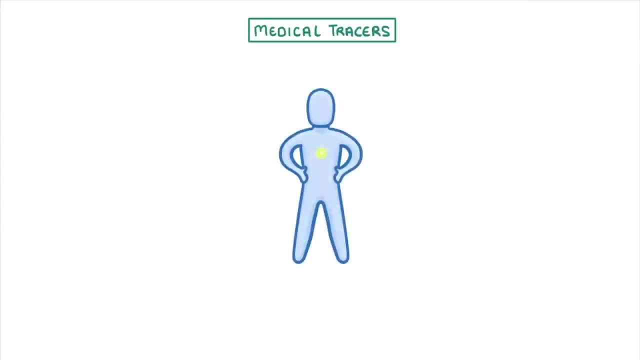 radioactive isotopes inside a person's body, which we can do by injecting them or getting the person to swallow them. then we can actually track the movement of the isotopes around the person's body by tracking the radiation that they emit. This means that we can actually 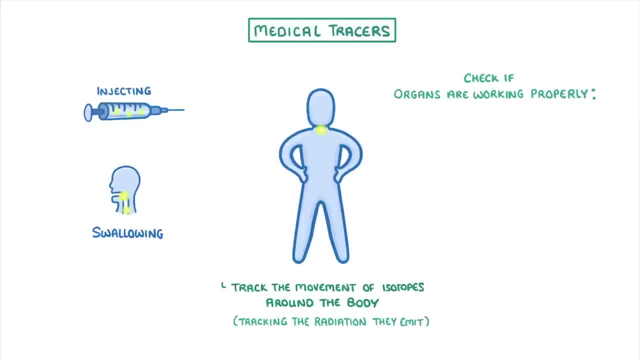 check if particular organs are working properly by seeing if they absorb the right amount of the substance. For example, by giving people iodine-123,, which means gamma radiation, we can see if the iodine is being absorbed by the thyroid gland like it should be, because 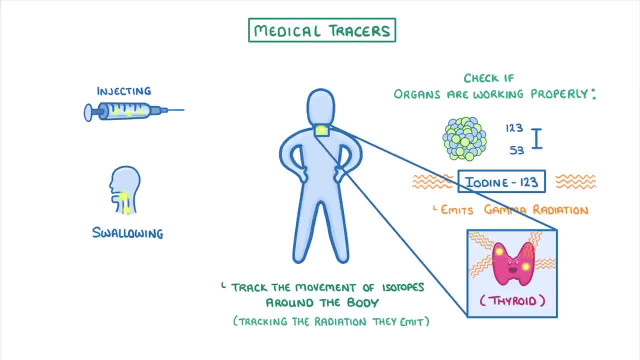 if it is, then we'll be able to detect the gamma radiation. We tend to use gamma rays for medical traces because they are less harmful than alpha or beta, Although we do sometimes use beta radiation. We also want to use isotopes with as short a half-life as possible, so that they only